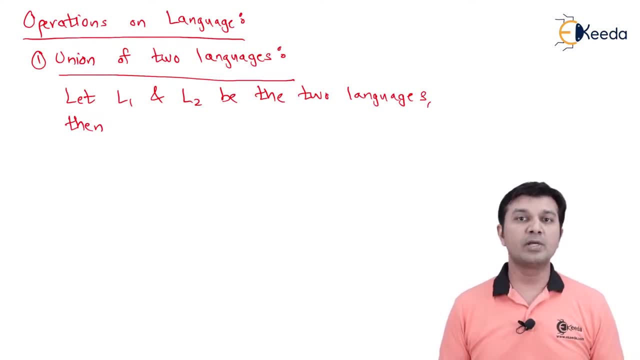 I'll be doing small examples on it and those examples will actually clarify the definition 100% to you. So right now, what is important is you understand the definitions as I say. So the first definition which we have over here is called as union of two languages. Now union operation is very simple. When I say union of two languages, the definition says let L1 and L2 be the two languages. Then L1- union of two languages. 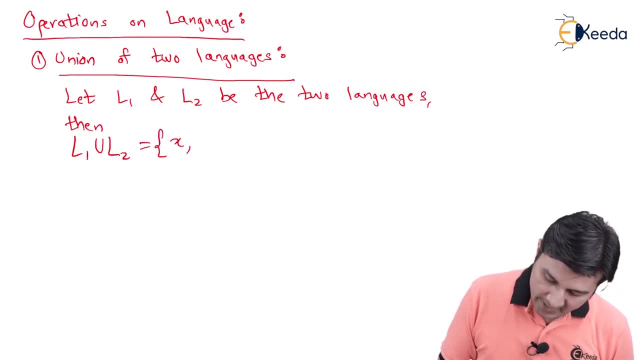 Then L1, union, L2 will be the set of all X, Y, Most important, we have a comma in between. That's where it is going to be distinguished from the remaining operations. So L1, union, L2 is set of all X, Y, such that X belongs to L1 and Y belongs to L2.. That is nothing but my union operation. So union operation simply says that pick up something from one set, Pick up something from another set. 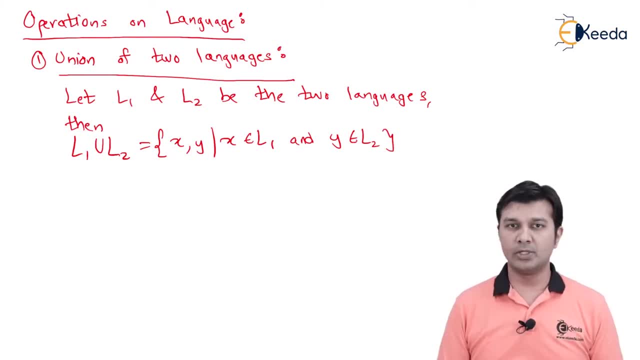 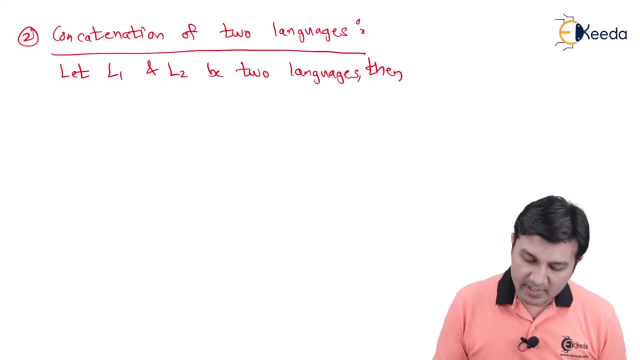 Join together, and that is my union operation. The next operation says concatenation of two languages. It is defined as: let L1 and L2 be the two languages. Then I say: L1, dot, L2 will be set of all X, dot, Y, such that X is going to belong to L1 and Y will be belonging to L2.. 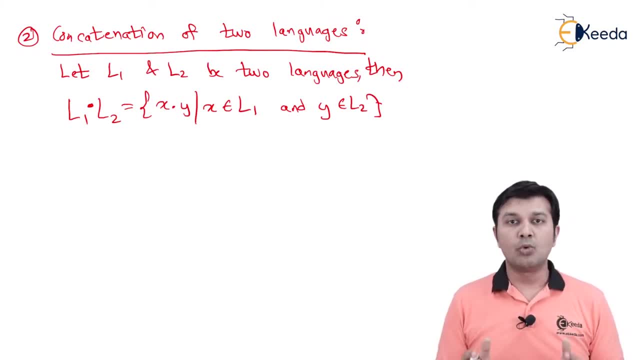 So L1 union, L2 was union. That is nothing but simply joining L1 and L2.. Whereas L1 dot, L2 is the concatenation operation, That is, everything in first set will be concatenated with each and everything one by one available in the next set. 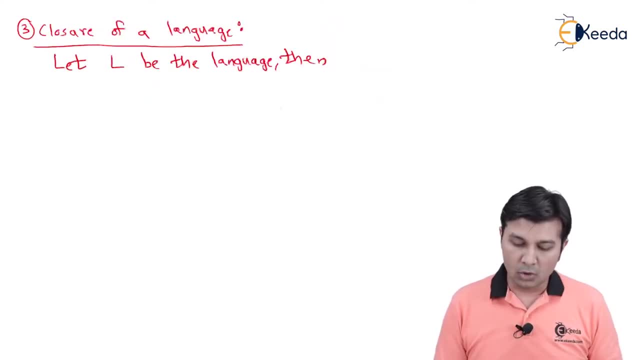 Going ahead. the next definition which we have is the closure of the language. Now for the closure. a very important property, because this is something that we are going to talk about in the next set. This is something that we are actually going to carry as a de facto standard throughout the syllabus. 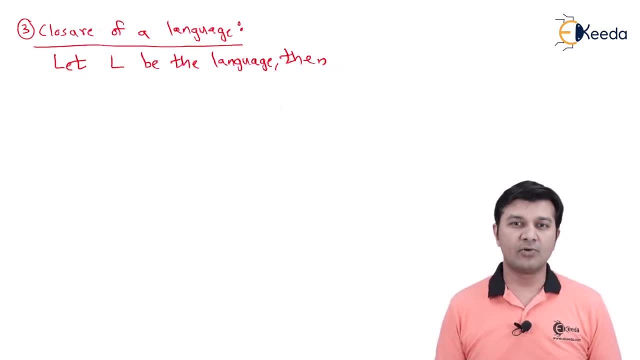 So we can consider more of it like a legacy for us, because this is something which will be repeated again and again, And if you don't understand the concept of closure, understanding everything after this will be a big problem. So I say: let L be the language. Then my L star is called as the closure of a language. 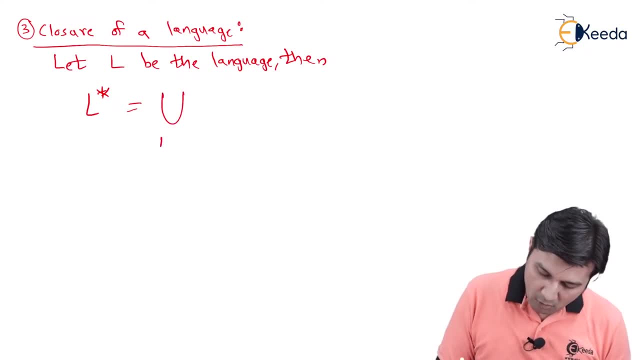 And it is defined as L dot, L2.. And it is defined as union of all the L? I's where I is going to go from 0 to infinity. What is important right now to understand before we proceed to the example, is the closure of the language is denoted by L star. 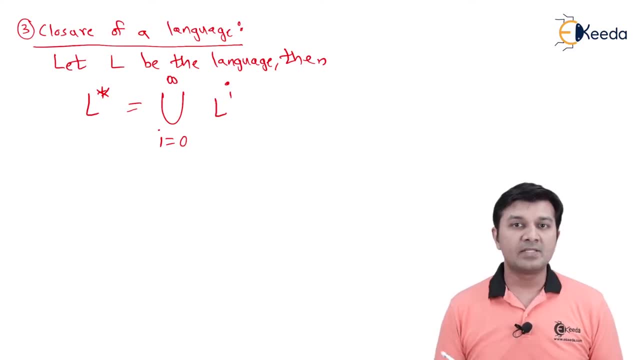 And it is set of all L I's where I is running from 0 to infinity. So what is important is it is denoted by L star And it is running From 0 to infinity. Let's go ahead to the next definition. 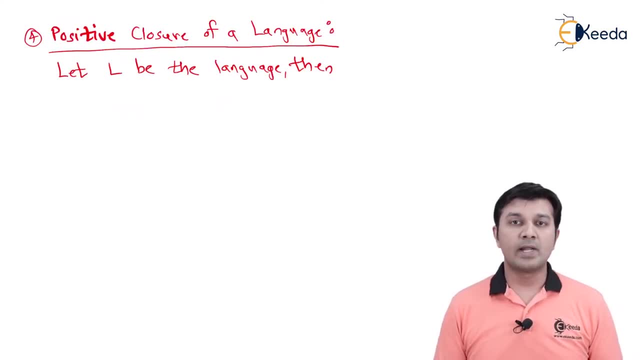 Following the closure, the next definition which I have is called as the positive closure of a language. Now the positive closure of a language is defined as: let L be the language, Then the positive closure- L plus, denoted by L plus, is again set of all L. I's quite similar to the previous one. 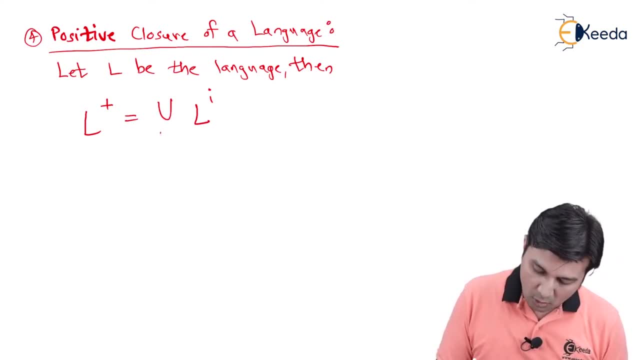 But over here this set of L? I's Is union of I is equal to something to infinity. Previously, this something was 0.. Now the only difference over here is the something is 1.. So positive closure is nothing but set of all L I's running from 1 to infinity and denoted by L plus. 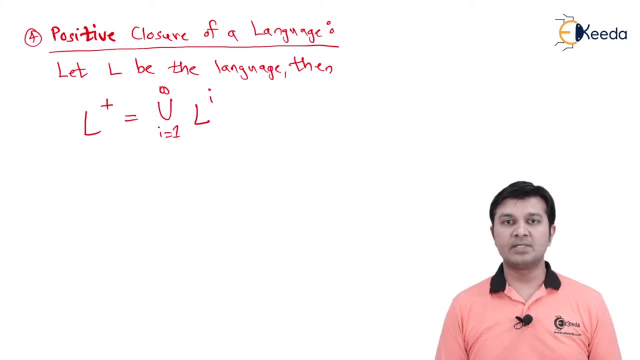 So these are the four operations on the languages that are important. So, summarizing these four operations, I say they are the first one, called as As the union, then concatenation, then closure and positive closure. Now let's understand how we can call it in the simplest name to remember. 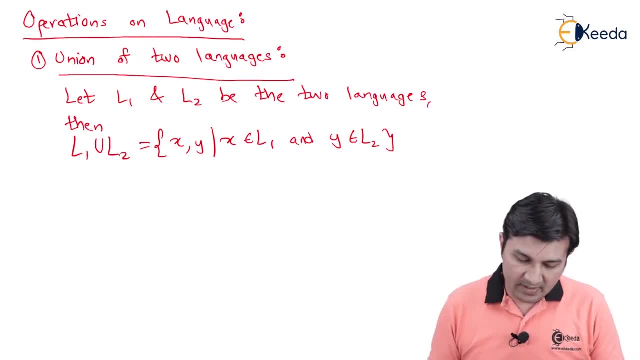 So, moving on to the first operation, that is union. So I say, whenever I talk of union, I say I will never look for a combination. Remember this is very important: Whenever I talk of union, I never look for combination. The next definition: concatenation. 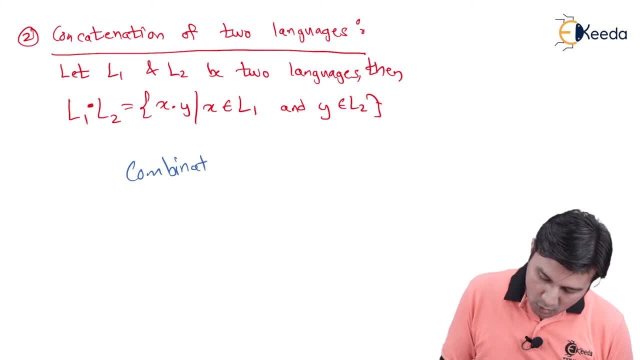 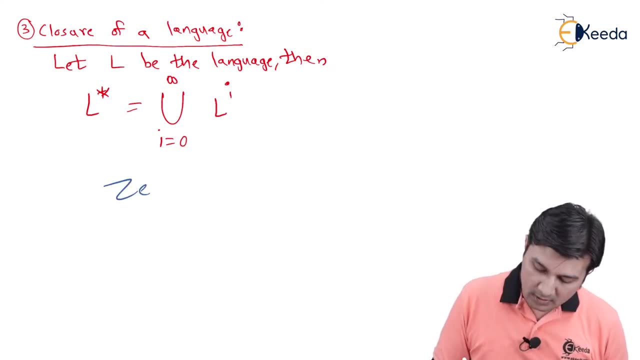 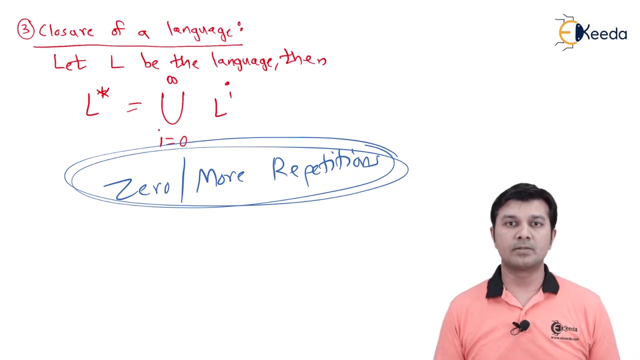 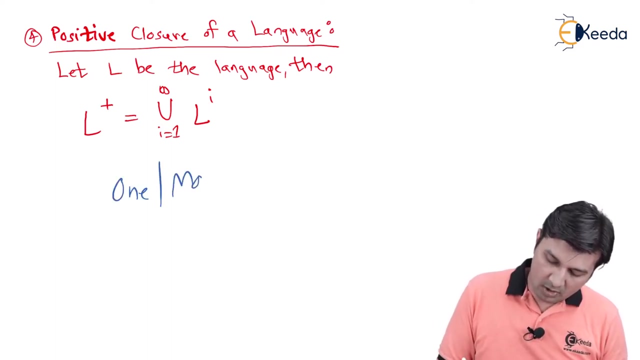 Whenever I look for concatenation, I am looking for the combinations. The next definition: closure. Whenever I talk of closure, I am looking for zero or more Repetitions and the last one, positive closure. When we talk of positive closure, I am looking for one or more. 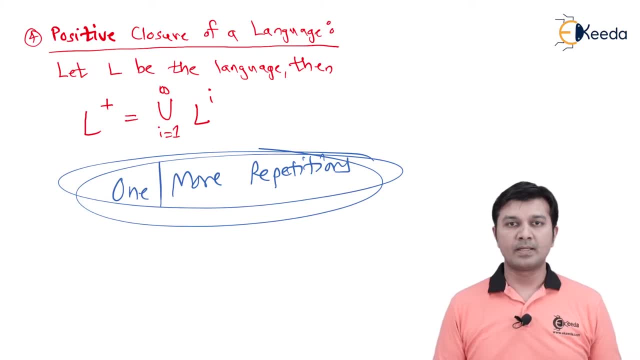 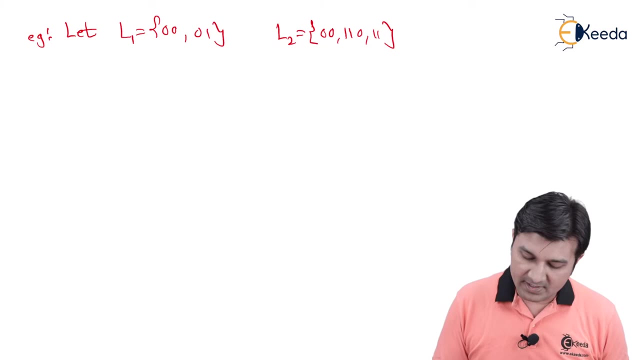 Repetitions. So, having completed the definition, let's look a very small example on it so that we understand 100 percent of it. So we have over here my languages stated as follows: I have my L1 given as zero, zero, zero one. 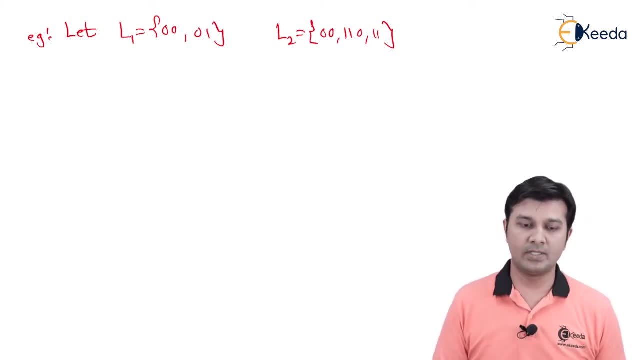 I have L2 given as zero, zero, one one zero and one one respectively. So if I say I want to find the first operation, that is L1 union L2.. It is merely joining L1 and L2.. So L1- everything will be coming over here. 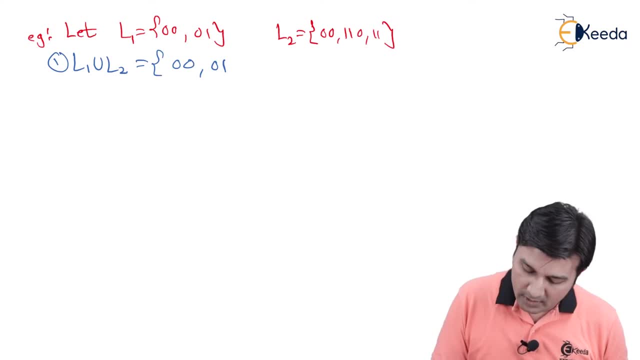 That is, L1 has zero zero and zero one. We grab it over here among L2.. We have zero zero, But we see that zero zero is already a part of it. Therefore, we ignore that And I take the next one as one one zero and the next one as one one. 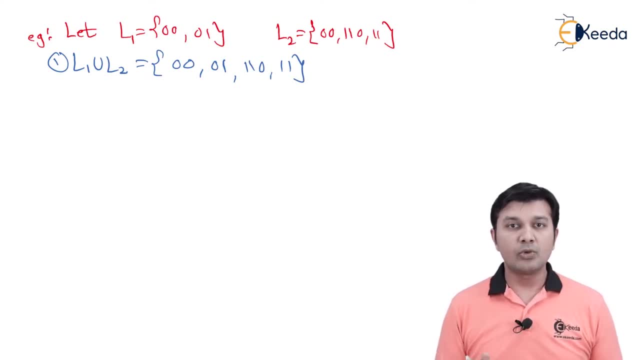 That is nothing but my union operation. Therefore I say, in union we don't look for combinations. The next one, the next operation which we have is L1- dot- L2.. If I talk of L1- dot- L2, I will be initially taking L1's first string, that is zero, zero. 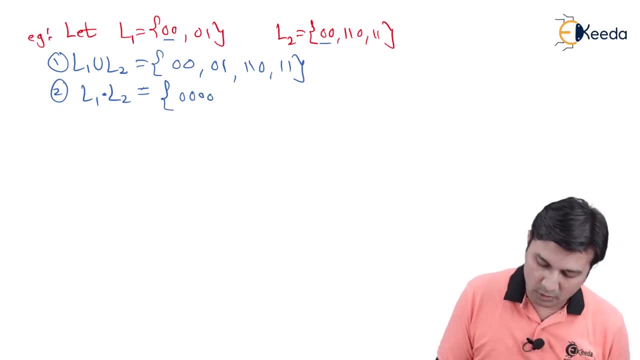 and appending it with L2's first string, that is zero, zero. So the number which I get over here is zero, zero, dot, zero, zero, which is nothing but zero, zero, zero, zero. Again, I take zero, zero from L1 and I append one one zero ahead of it and I get this string. 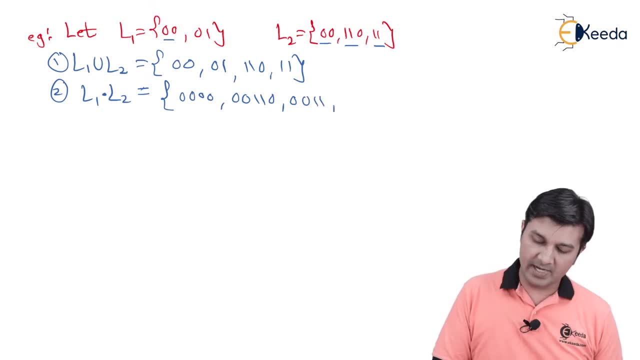 Again, I take zero, zero, append one one ahead of it. I get the third string going ahead. This time I will be taking zero one from L1 and appending it with zero, zero of L2.. Again, I take zero, one of L1. 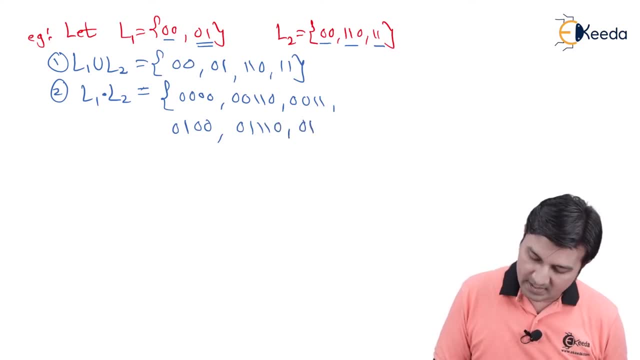 and append it with one one, zero of L2. and lastly, zero one of L1 appended with one one of L2.. That is my concatenation operation. So whenever I talk of concatenation operation, I am basically looking for combinations. So now you can understand, when I say L1 and L2, why I used to say it is nothing. 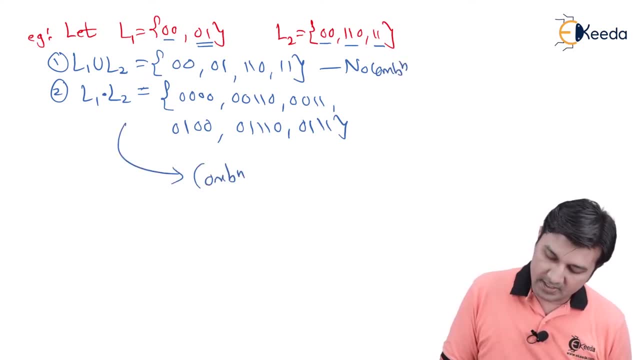 but no combination. and L1, dot, L2 is nothing but looking for only combinations. The next part of the definition, the third one we are looking for, L star. that is nothing but the closure of a language. For that, let's go to the new slide first, so that we can start afresh. 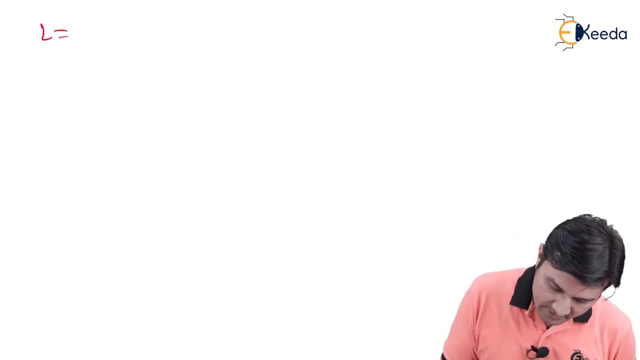 So we have over here our L given as AB. Now, whenever I say L is given as AB, if I say what is going to be my L2, my L2 is going to be nothing but L1, dot, L1 and L1, dot, L1 is nothing but taking AB twice. 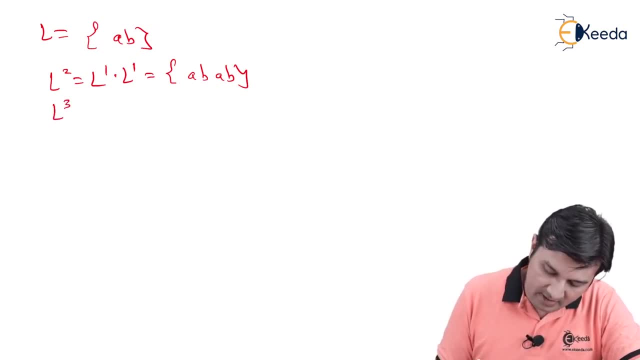 Similarly, if I say: what is L3,, L3 is going to be nothing but L1, dot, L1, dot, L1, which is nothing but taking AB thrice. Similarly, if I say: what is L1 in that case? L1, in that case is: 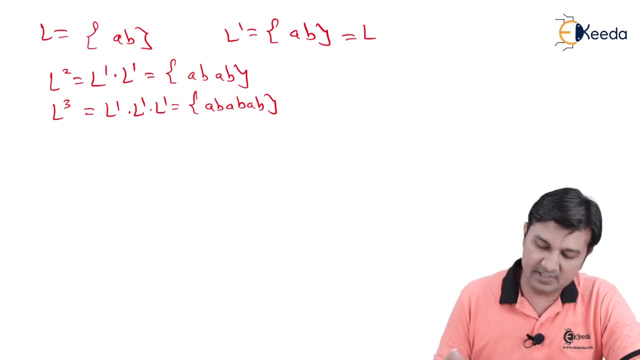 nothing but taking AB. thrice, Nothing but taking AB. So I can also say: L1 is as good as L. So I have my L1 with me, I have my L2 with me, I have my L3 with me. Similarly, I can say my L4 will be equal to AB, AB, AB, AB. four number of times. 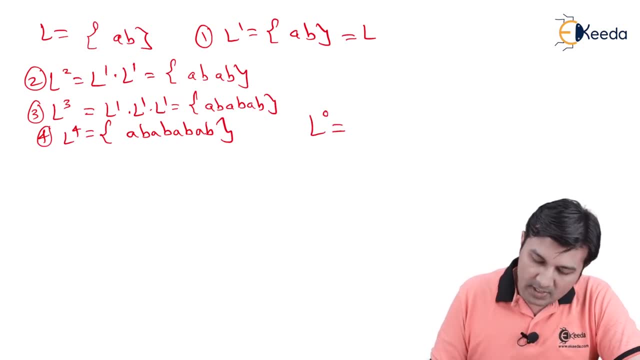 What is my L0 going to be? My L0 is going to be nothing, but no input to be taken from the set AB. So since no input is to be taken, we never write it as zero in automata theory. We just discussed it in the previous topic. 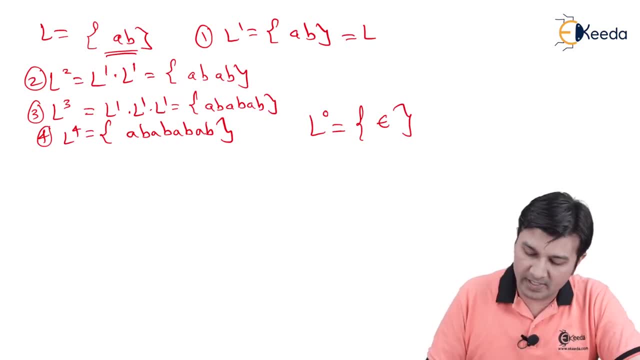 Spring of length. zero is denoted by epsilon and therefore we write: L0 is equal to epsilon. If now I see what is going to be my L star, we all know that L star is nothing but the union of I, equal to zero, to infinity of all LIs. 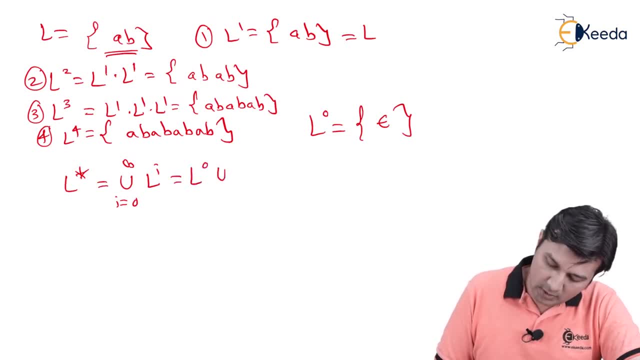 So can I say it is nothing but L0 union, L1 union, L2 union, L3 union, L4, so on and so forth, up to L infinity, And we all are very much acquainted with the operations of union. When I say what is union of L0, L1, L2 up to infinity, it is merely joining all those things or creating no combinations of it. 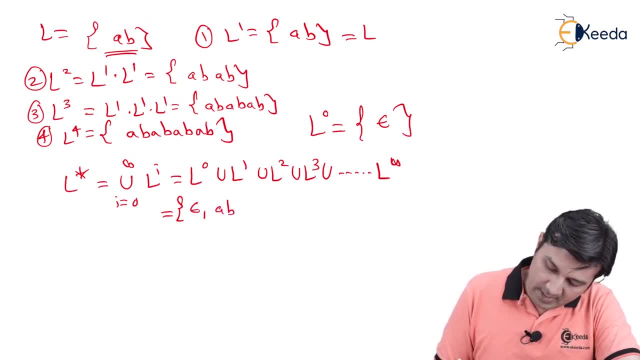 So I say it is going to be nothing but epsilon, AB, AB, AB, AB, AB, AB, so on and so forth up to infinity. So if I look at this particular example, can I typically conclude that my L star is: 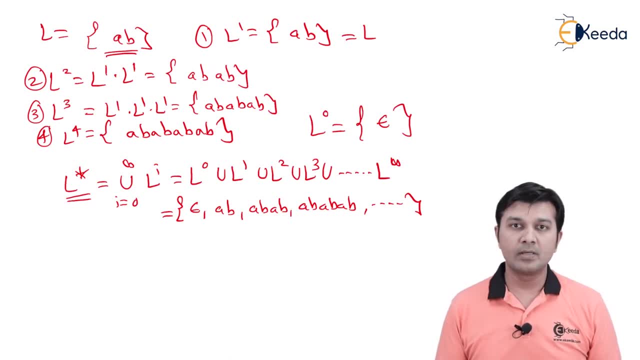 nothing but zero or more repetitions of AB. Exactly That's what my L star means And that's exactly what we wrote across the definition. It is meaning zero, Zero or more repetitions. So if I say the input string given to me is CA, and what is L star? 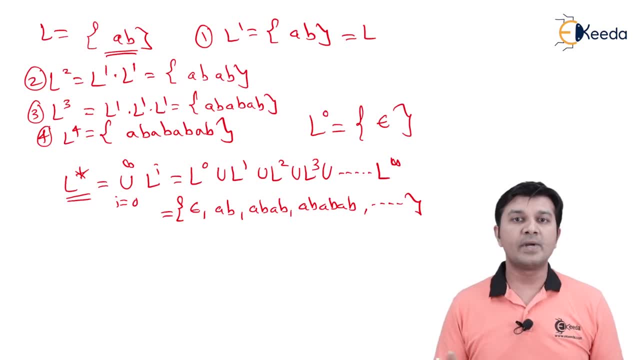 The only answer to it is: it is zero or more repetitions of CA, So the language will have strings like epsilon: CA, CACA, CACACA, so on and so forth till infinity. Remember: CA taken twice doesn't become CCAA. 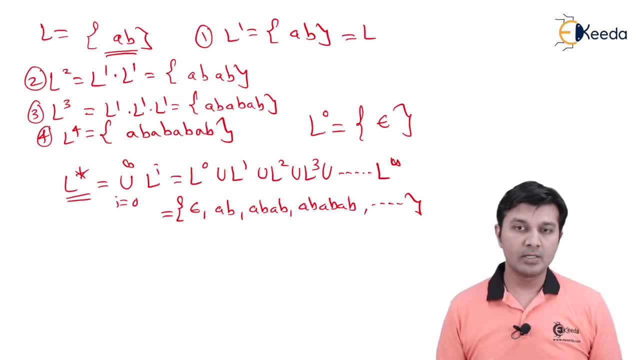 So the output string has to maintain the order. Similarly, the fourth definition which we are talking of, L plus. L plus was called as the positive closure. So the only difference compared to the previous one over here is it is one or more repetitions. 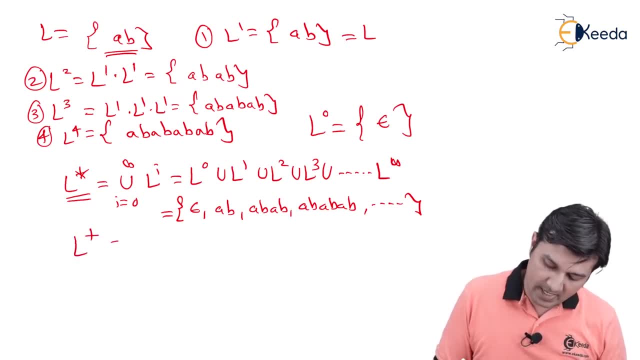